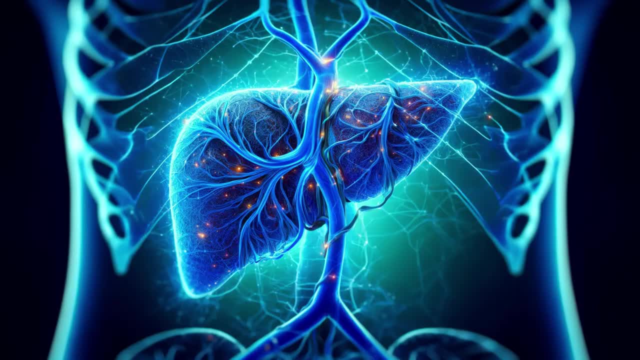 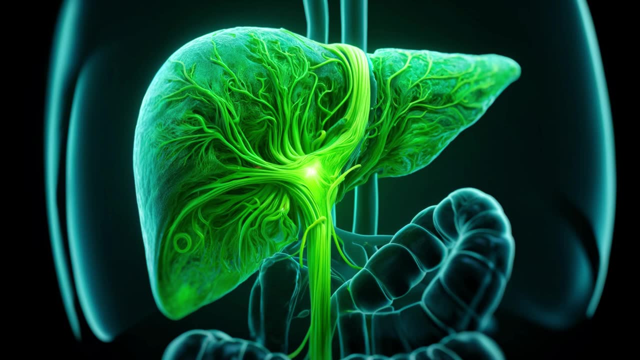 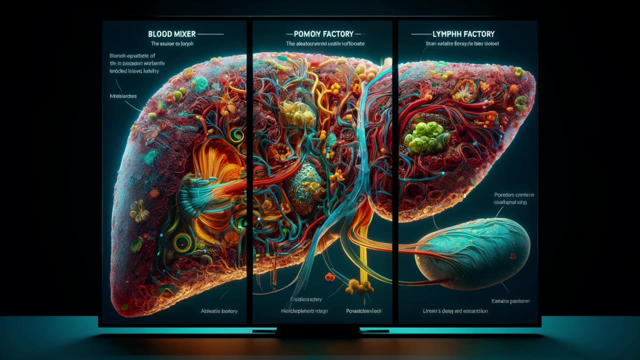 trove of nutrients absorbed from our food and the intestines Bile duct. This is the waste disposal system: transporting bile, a greenish-yellow fluid the liver produces, away toward storage and later use. The space of Maul isn't just about transportation, It's a multitasking powerhouse. Let's break down. 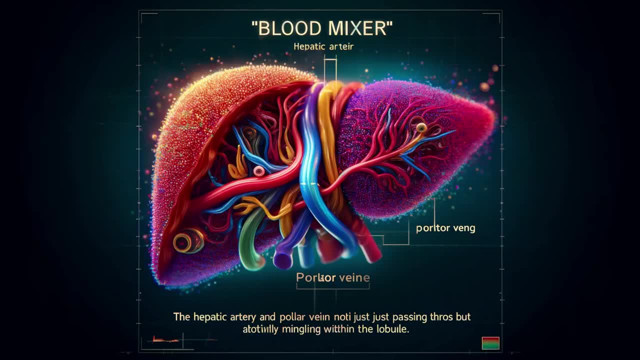 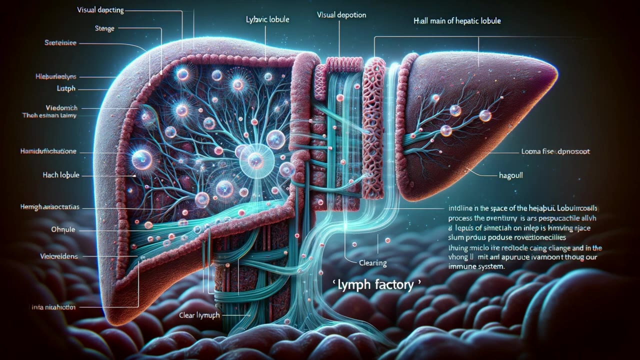 some of its key functions: Blood mixer, The hepatic artery and portal vein don't just pass through, They mingle and exchange precious cargo here. This ensures an optimal blend that nourishes the busy hepatocytes. Lymph factory- Lymph- a clear fluid vital for our immune system. 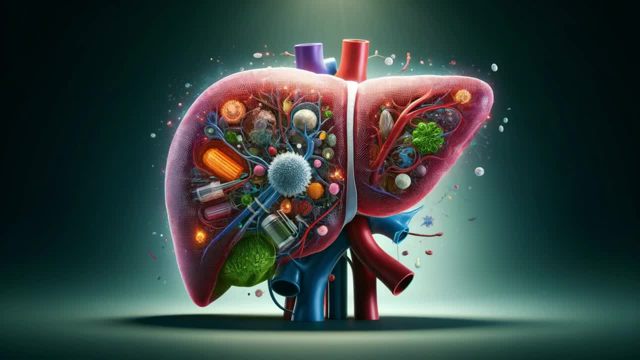 is also produced within the space of Maul Liver's detox center. The liver is a giant filtration plant. Within the space of Maul, blood is meticulously cleansed. Toxins like alcohol, drugs and other harmful substances are captured and transformed to. 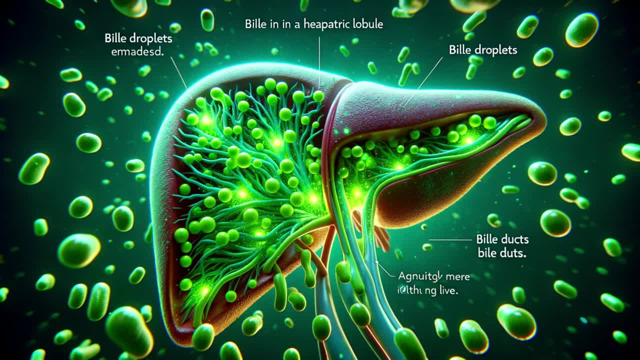 protect our bodies. Bile, essential for fat digestion, doesn't just vanish. The space of Maul is where the bile collection network begins: Hepatocytes, secrete bile, which flows into intricate bile ducts. As these ducts merge, carrying their precious cargo. 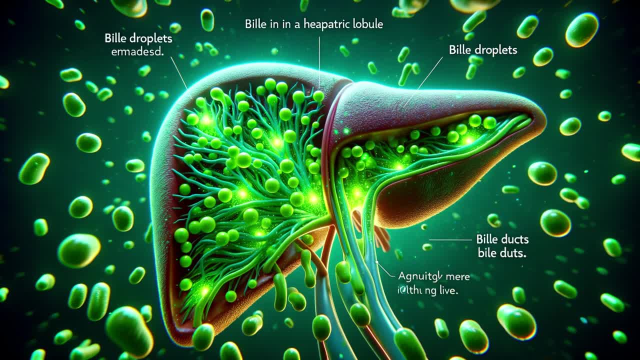 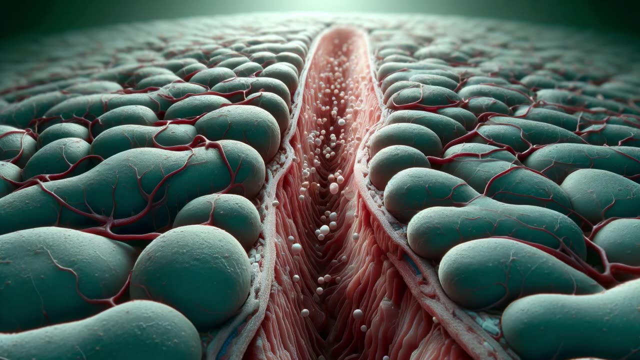 they form a network mirroring the branches of the hepatic artery. This ensures maximum exposure to the fresh oxygenated blood for a boost before traveling on to the gallbladder or directly to the intestines. Zooming in even closer, we discover a hidden marvel: the space of dis, This minuscule 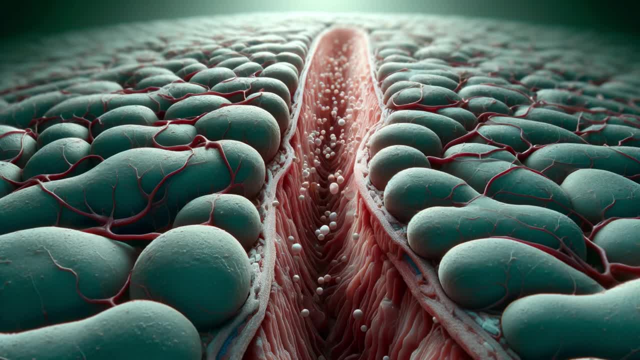 space between individual hepatocytes and blood vessels is the ultimate delivery zone. Think of blood vessels here as leaky pipes with tiny perforations. Through these nutrients, oxygen and other vital substances can be produced. The blood vessels are the ultimate delivery zone. 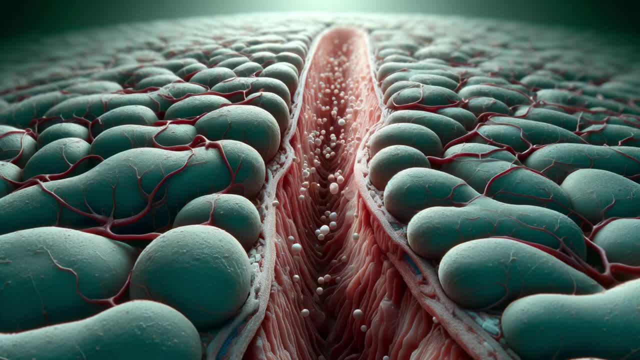 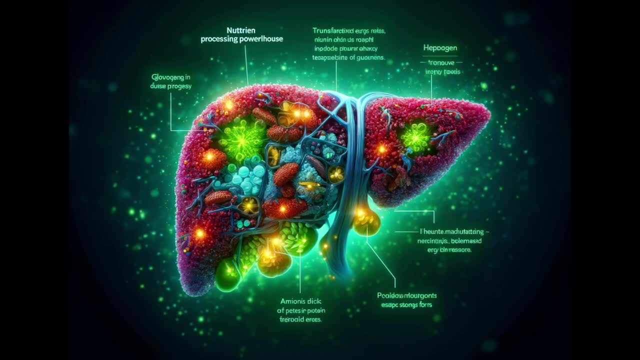 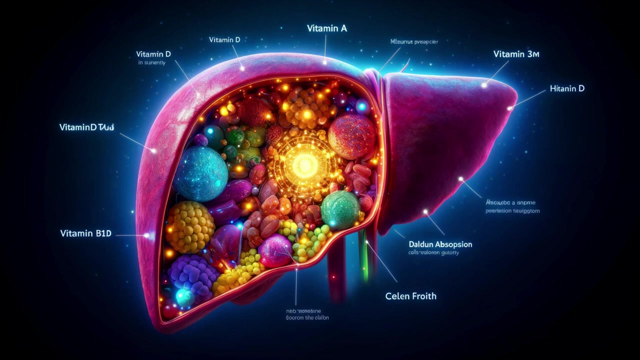 Nourishing hepatocytes directly. It's like room service for the liver's hard-working cells. They also manufacture amino acids, the building blocks of proteins essential for building and repairing tissues throughout our body. Vitamin Volt glowing yellow. Our bodies rely on a steady 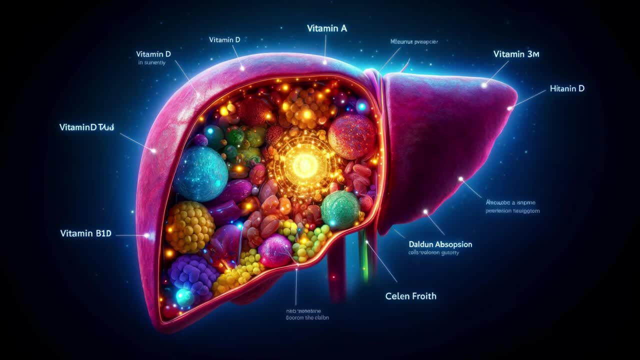 supply of vitamins to function properly, The liver acts as a vital stockpile, particularly for vitamins A, D and B12.. Vitamin A, highlighted in glowing yellow within the cell, is crucial for vision, immunity and cell growth. Vitamin D, another glowing resident, helps regulate calcium. 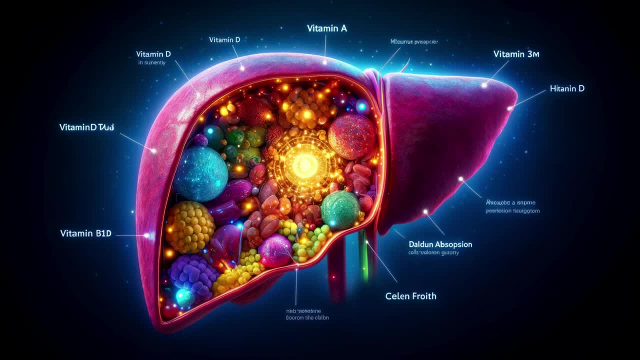 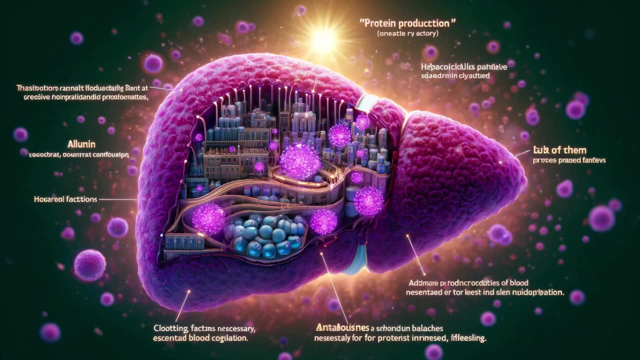 absorption for strong bones and teeth. Finally, vitamin B12, a glowing blue orb, plays a key role in red blood cell production, nerve function and DNA synthesis. Protein Production Factory. Glowing Purple Hepatocytes are like tireless manufacturing plants when it comes to protein production. 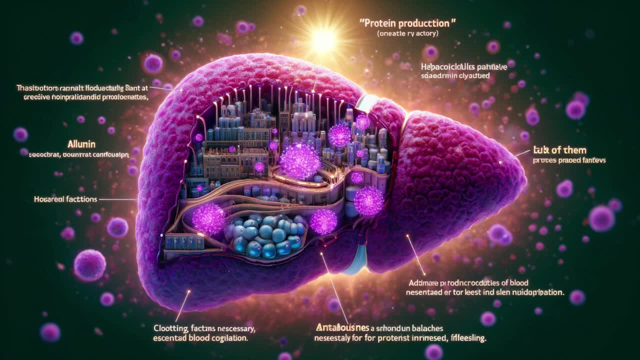 They churn out albumin, a glowing purple protein that helps maintain fluid balance in our body, preventing swelling. They're also responsible for crafting clotting factors, essential for preventing excessive bleeding and inflammation After injuries. and let's not forget their contribution to our immune system. 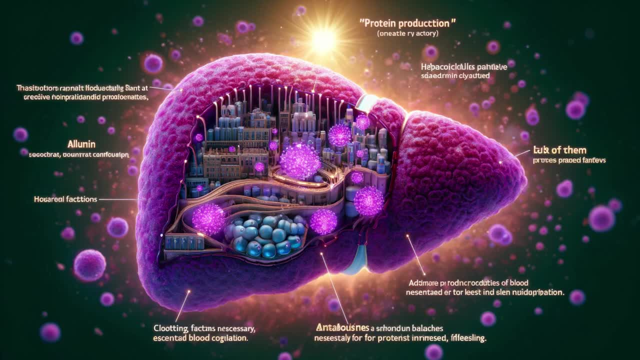 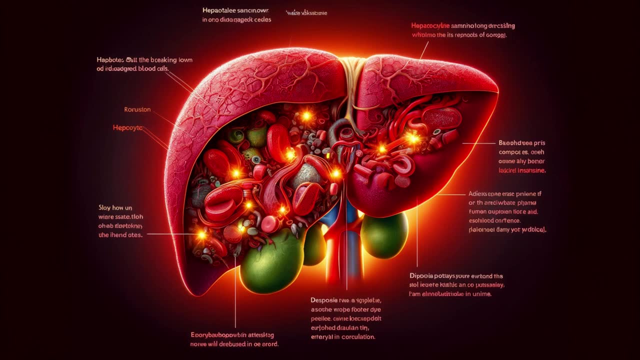 Hepatocytes produce antibodies: glowing purple, defenders that fight off infections and keep us healthy Waste Management Center glowing red. Our bodies constantly produce waste products. Hepatocytes act as the liver's sanitation crew, breaking down old or damaged red blood cells. 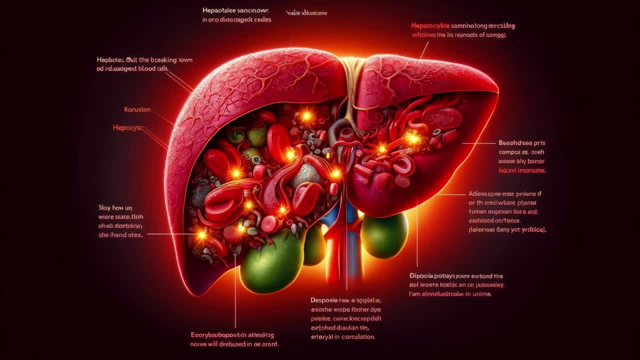 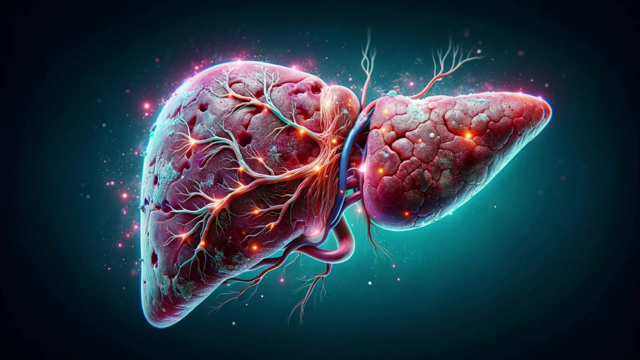 They meticulously recycle iron and other useful components from these cells, returning them to circulation. The remaining waste products are either disposed of through bile or filtered out by the kidneys for elimination in urine. Beyond its daily grind, the liver possesses a remarkable secret weapon: regeneration. 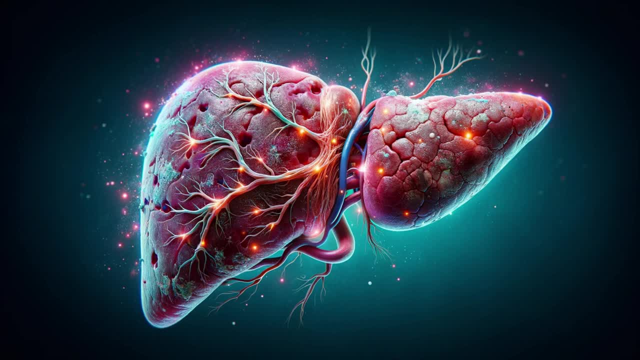 It's one of the few organs that can regrow, replacing damaged tissue. This resilience is crucial for overcoming injuries or the impact of certain diseases. The liver's regenerative abilities are truly awe-inspiring. Even if a significant portion of the liver is damaged, the remaining healthy cells can kill the liver. Even if a significant portion of the liver is damaged, the remaining healthy cells can kill the liver. Even if a significant portion of the liver is damaged, the remaining healthy cells can kill the liver. The liver's regenerative abilities can kill the liver. 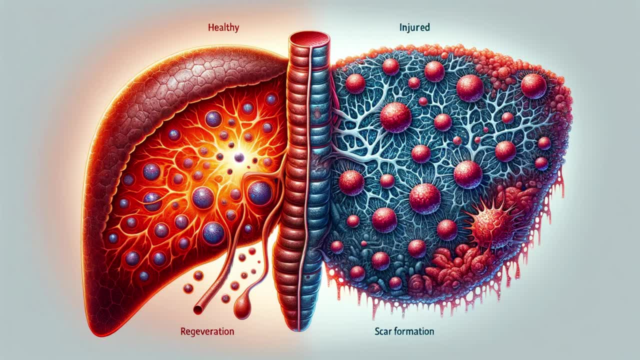 In this process, one uses its own physical function and the would Miller instrument to make things easier. This process called hepatic regeneration allows the liver to restore itself and regain full function. This process called hepatic regeneration allows the liver to restore itself and regain full function. 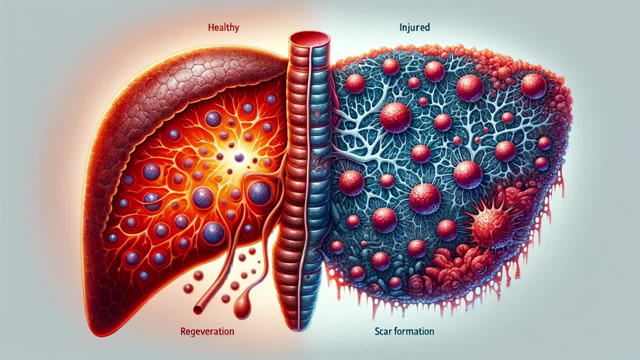 This remarkable feat is facilitated by the presence of special precursor cells that act within the liver, called hepatic stellate cells, and are �ceran cells Within the liver called hepatic stellate cells. In a healthy liver, these cells are quiescent, focusing on storing vitamin A. 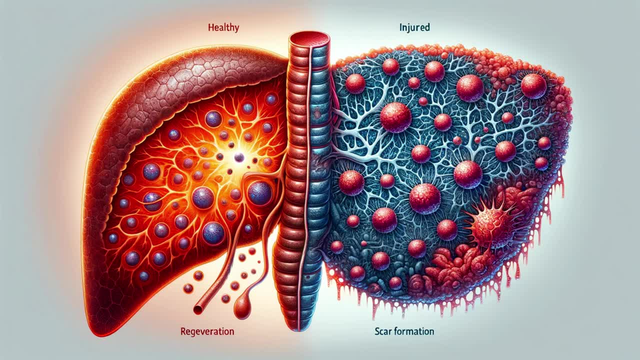 In a healthy liver, these cells are quiescent, focusing on storing vitamin A. However, when the liver is injured, these cells become activated and transform into scar-forming myofibroblasts, While scar tissue is necessary for initial rejuvenation. 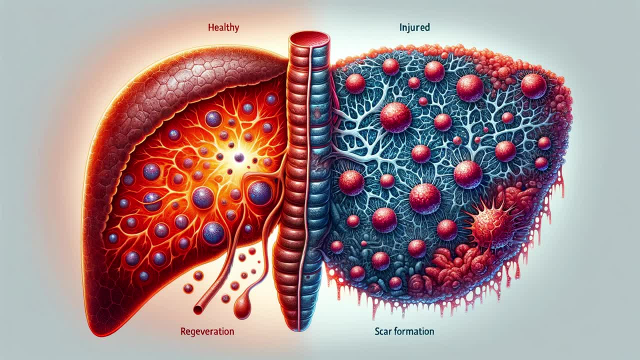 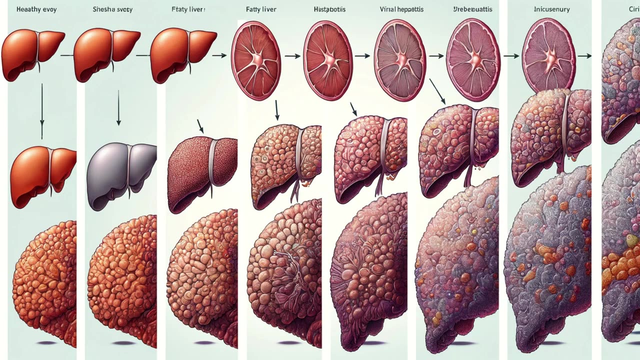 for initial healing. excessive scar tissue buildup, known as cirrhosis, can hinder the liver's ability to function properly. Understanding the delicate balance between regeneration and scar tissue formation is key to developing new treatment strategies for liver diseases. Unfortunately, our liver's amazing abilities have limits: Poor, diet, excessive. 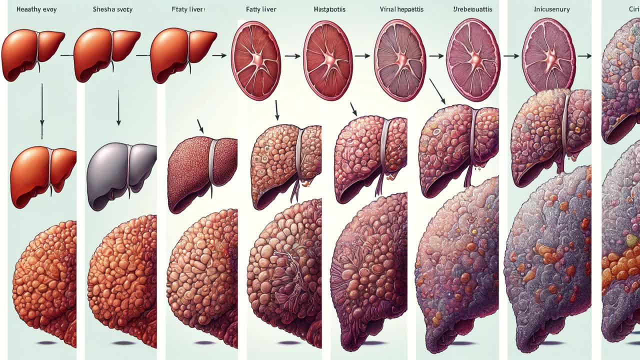 alcohol, infections or other underlying conditions can overwhelm the liver's defenses. The space of maul and space of dissey aren't immune. Scarring can disrupt blood flow, bile transport and hinder the liver's functions. This is why it's so important to care for this. 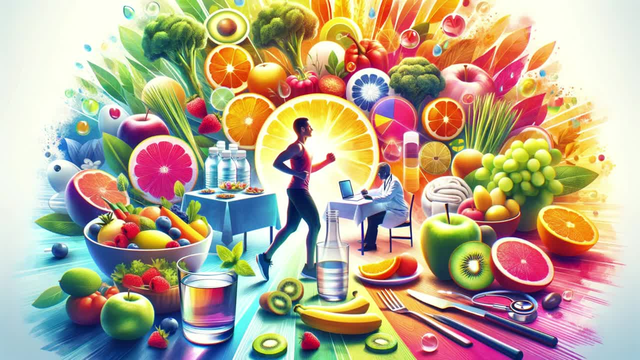 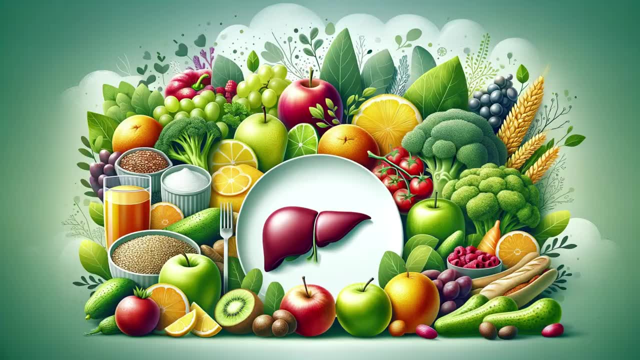 vital organ. The good news is, we can support our liver's health, ensuring those fascinating spaces keep functioning at their best. It's all about smart choices. Eat well. A balanced diet rich in fruits, vegetables and whole grains nourishes your liver. Limit fatty, sugary. 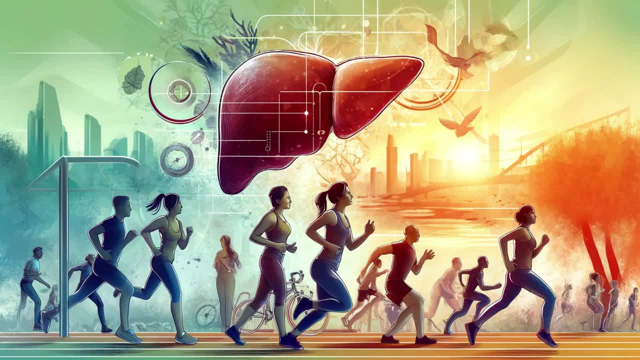 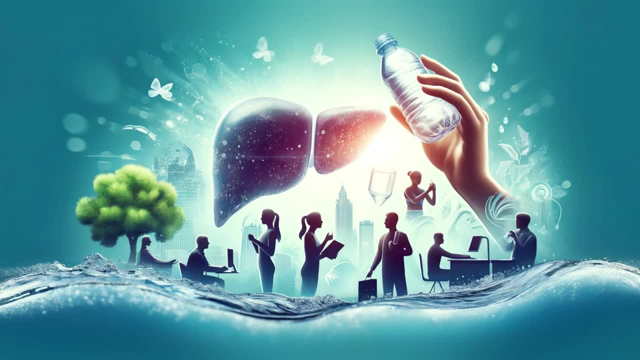 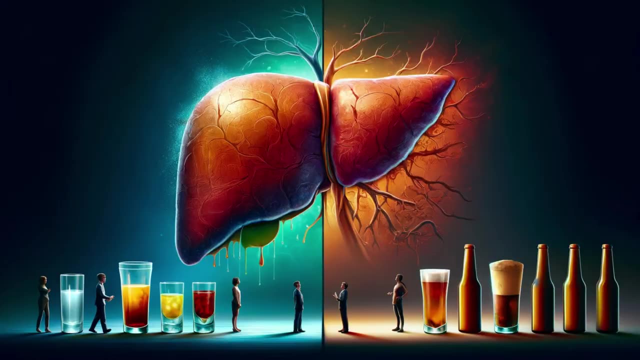 and processed foods. Stay active. Exercise helps maintain a healthy weight and reduces harmful fat buildup in the liver. Hydrate Water aids in flushing out toxins and supports optimal liver function. Limit alcohol. Overworking your liver with excessive alcohol takes a heavy toll. 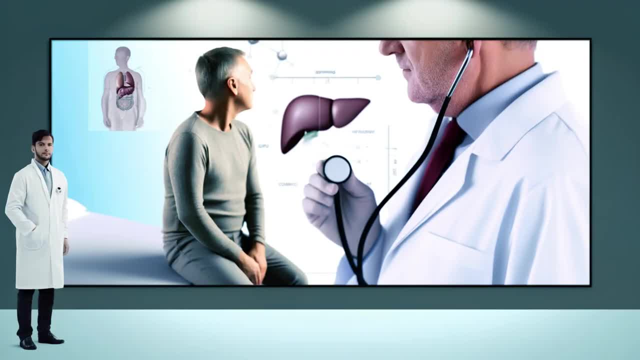 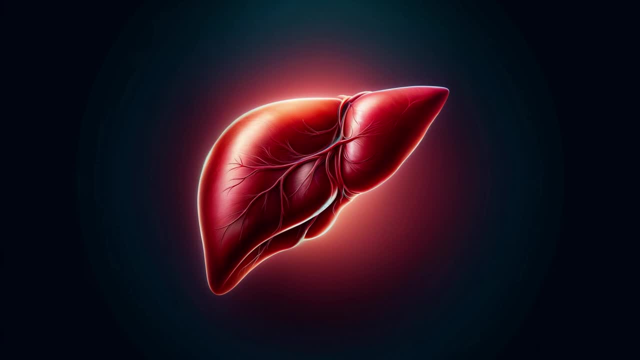 Get checkups. Regular checkups can catch liver issues early, when they're most treatable. The liver may toil in the background, but its impact on our well-being is immeasurable. From the bustling space of maul to the microscopic space of dis, this intricate organ structure ensures an incredible range of 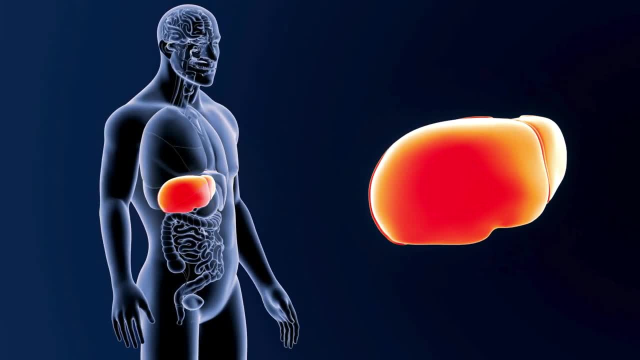 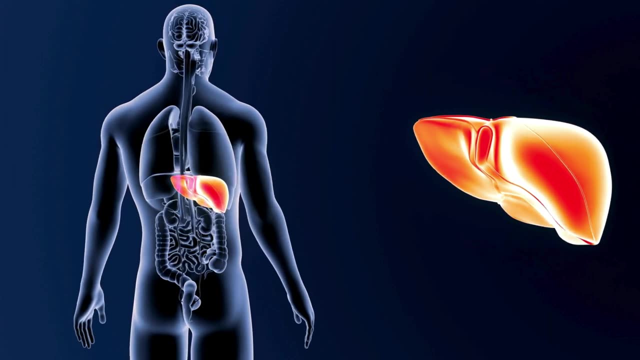 functions. Now, with this deeper understanding, let's pledge to treat our livers with the respect and care they deserve. After all, a healthy liver means a healthier you. Did this journey into the micro-world of the liver fascinate you? Let me know in the comments below. 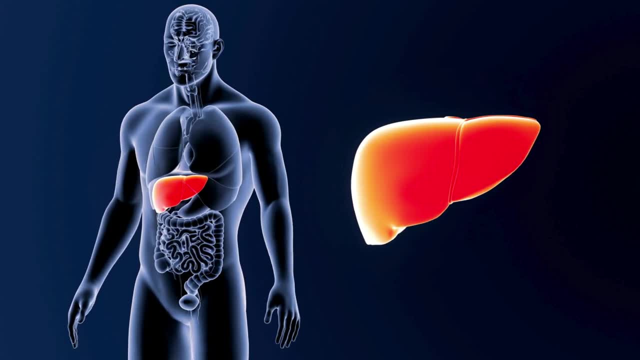 Don't forget to like and subscribe for more explorations into the wonders of the human body.